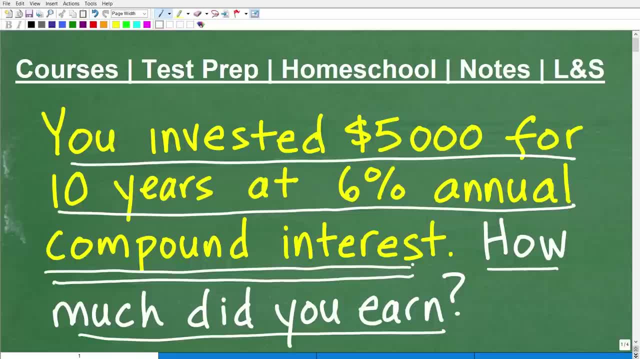 problem is this right here: compound interest. This is one of the most critical concepts that you have to understand, especially if you intend to invest. And to paraphrase Albert Einstein- I don't have the exact quote, but I believe he said something to the fact that the most powerful 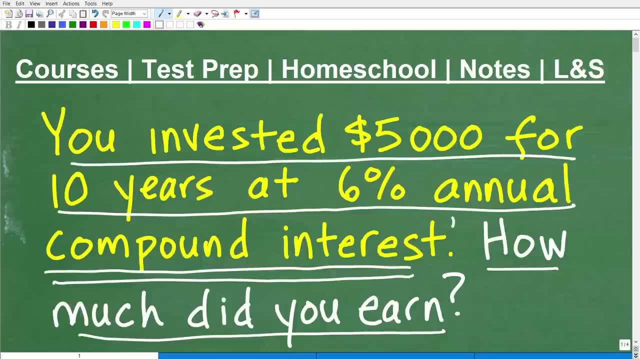 force in the universe is compound interest, Because compound interest goes to a concept in mathematics called exponential growth. Okay, this is an exponential growth function And if you understand this, we're going to give this problem a try. I'm going to put your answer into the comment section. A couple of things here. 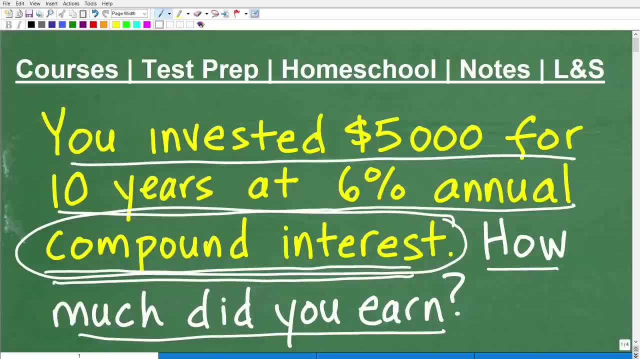 you're going to need a calculator and you're going to need the correct formula for compound interest. Probably most of you out there may or may not remember the formula, but you may not even know it. So if you want to look it up and try to figure this problem out, go ahead and do so. 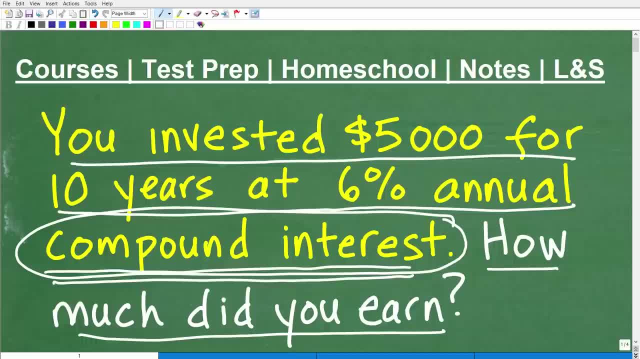 Just be careful, because there is a few different formulas for compound interest, And I'll talk a little bit more about that in a second. But before we get going, let me quickly introduce myself. My name is John. I'm the founder of TC Math Academy. I'm also a middle and high school math teacher. 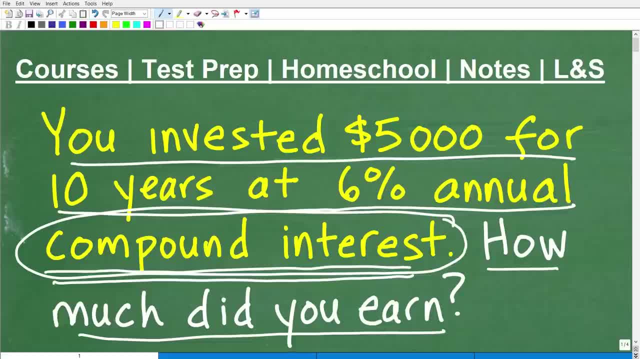 I've been teaching math for decades. I absolutely love teaching math And I can tell you right now, all of you could be successful in math, And I'm especially speaking to those of you that don't like math or you struggle in math. Okay, It doesn't have to be that way, Okay, So 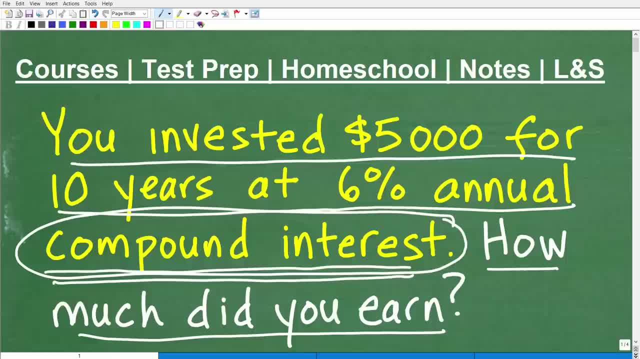 if you want to learn math, what you need is encouragement And, most importantly, you need great math instruction- instruction that you actually understand. So if you need help in your current math course, or maybe you're getting ready for some sort of special test that has 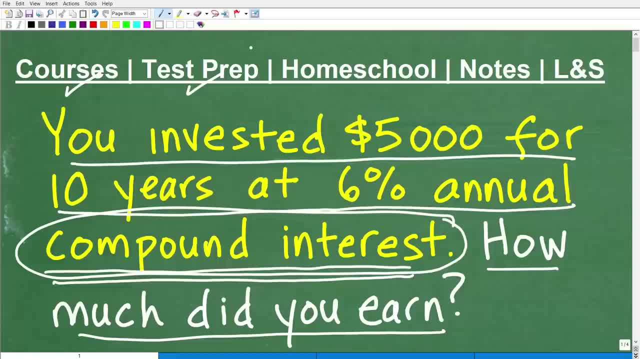 math on it. I'm talking about things like the GED, SAT, ACT, ASVAB, maybe a teacher certification exam or, if you're homeschooling mathematics, check out my math help program. I'm going to leave a link to. 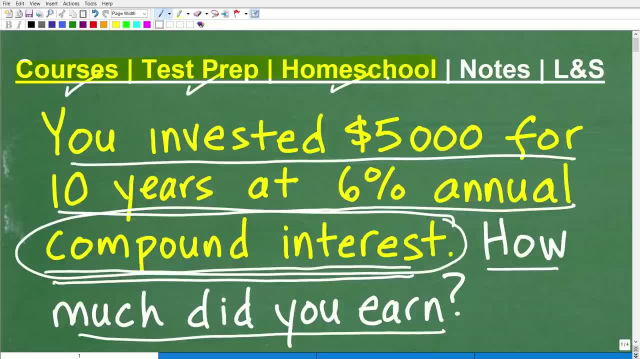 have over a hundred plus different math courses that span these categories and much, much more. I'm also going to leave links to my notes in the description as well, because a lot of students are not taking adequate notes. Some of you out there may not be even taking any notes, and that's a big 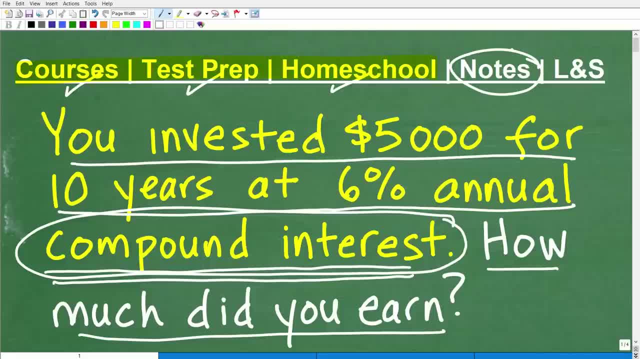 no-no in math. If you really want to do well in math, you have to be a great note taker, but you can use my notes in the meantime, And if this video helps you out, don't forget to like and subscribe, as that definitely helps me out. Okay, So let's go. 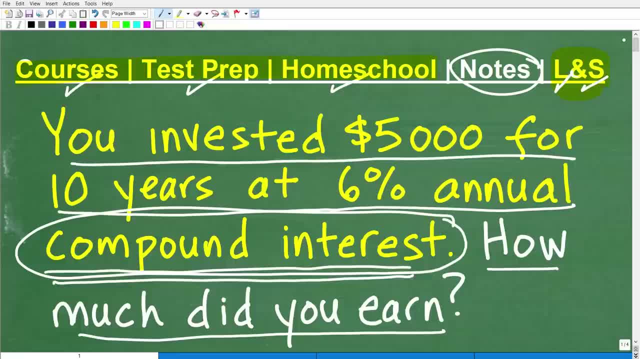 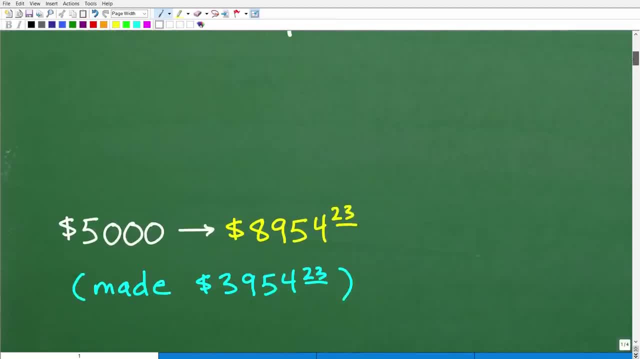 Let's take a look at the answer to this problem. So if you invested $5,000 for 10 years at 6% annual compound interest, how much money did you earn on that investment? Well, here is the answer. So our $5,000 grew into $8,954.23.. So that means you've made $3,954.23.. So you got to be careful. 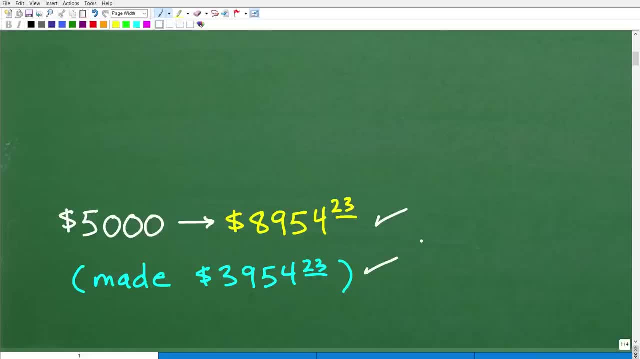 on your answers If you're saying: how much did you make? Well, you made this amount. Okay, This is your total account balance, but remember you started with your own money of $5,000.. So you made $3,954.23.. So your account. 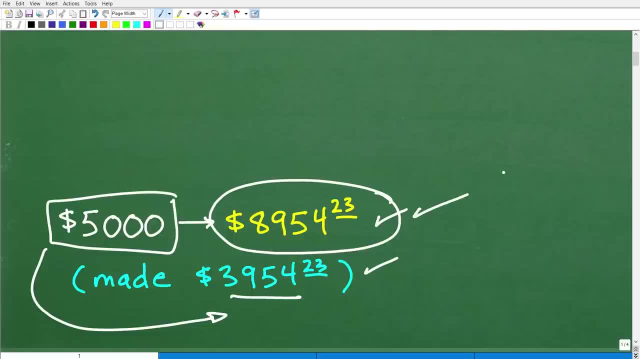 balance would be $8,954.23.. So we've got to be careful with what the correct question is asking. But if you gave me this answer, I would go ahead and still give you a nice, happy face, An A plus a 100% and multiple stars to celebrate your success in understanding compound interest. 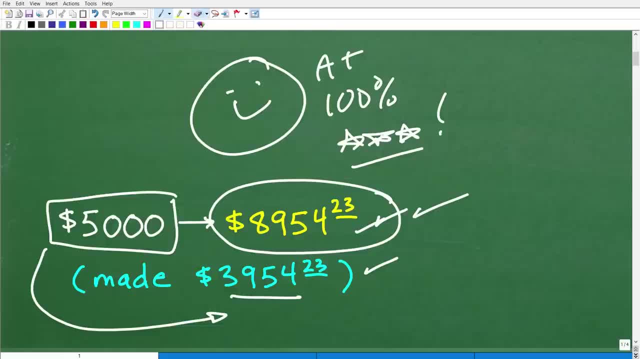 So again, as Albert Einstein was talking about some, maybe a hundred plus years ago, you know he knew back then that exponential growth is tremendously important. So compound interest is what we call exponential growth. Let me just kind of talk about this real, real quick, not to get overly. 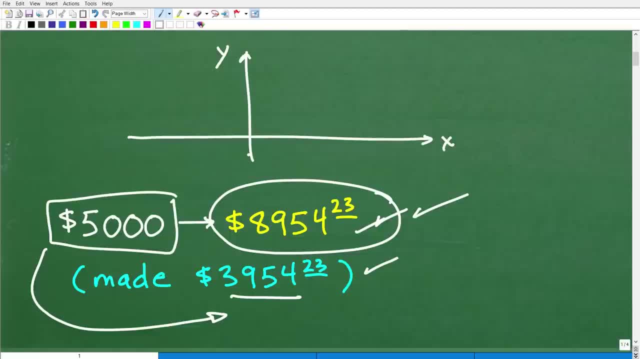 Technical here, but X there's basically is two concepts, something called exponential growth and decay. but exponential growth is something that looks like this: Graphically speaking, it kind of starts off some you know you have something that's kind of growing. 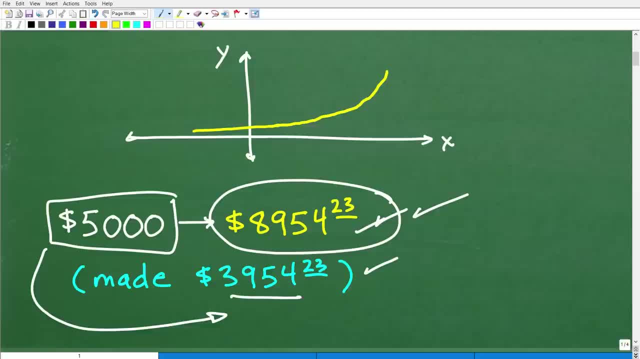 slowly, slowly, but over time it starts picking up momentum and it starts kind of shooting up this way. So this is what could happen in your investments- And you- all of us have heard this- Hey- if you put in like a hundred bucks a month into your IRA or 401k, if you do this for 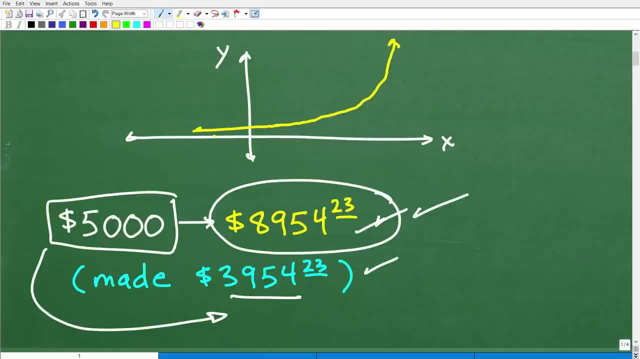 you know, years and years and years and years, it starts to really build up momentum. Well, what we're talking about is exponential growth, or compound interest, And it is true, all you know. this, of course, is assuming that you're getting a consistent, um you know, growth rate, a certain 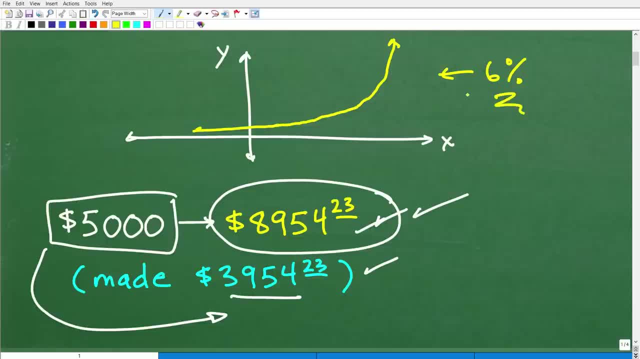 percentage. And this is the kind of tricky part when you invest. but if you do have a consistent um growth percentage, what ends up happening is, over the years, you know you're, you're kind of making a little bit of money And as you can kind of, you know, as time goes by, you know you're. 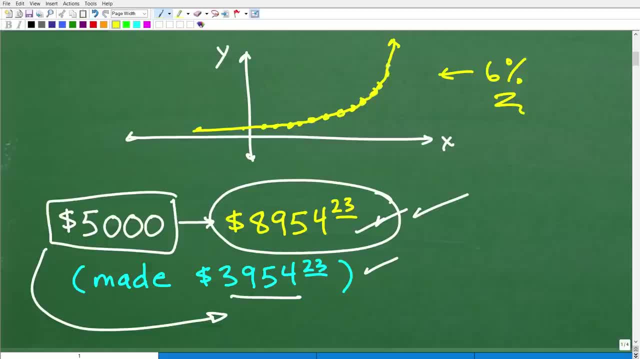 it starts to really pick up pace. So this kind of explosion in growth, this is what we call exponential growth And that's what compound interest is. Now this is a much bigger topic in mathematics: exponential growth and decay, which, of course, compound interest is a part of. 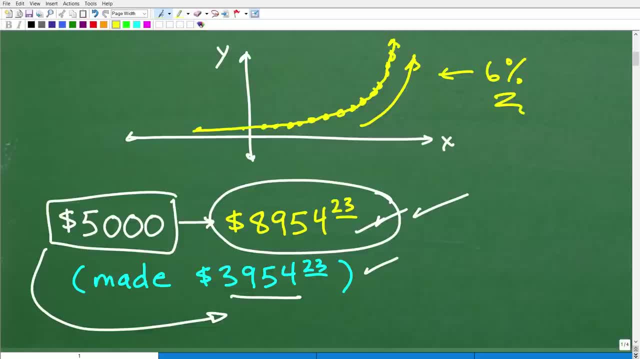 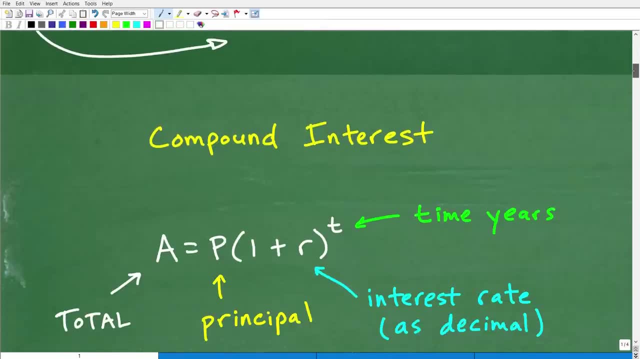 that, but I just want to make sure you understand why compound interest is so powerful. Okay, So let's go ahead and get into the specifics of this problem. So again, we have to talk about compound interest. So let's go ahead and get into the specifics of this problem. So again, we have to talk about compound interest. 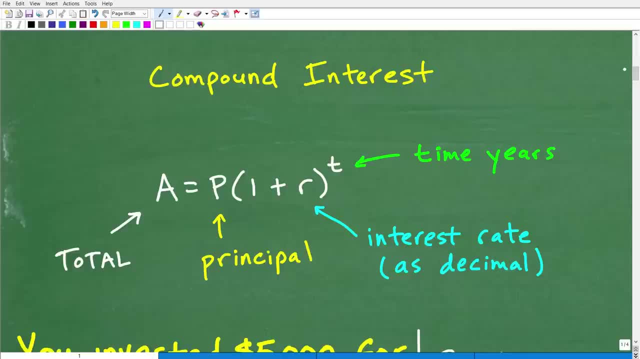 And we need a formula. Okay, So there are different formulas, a few different variations of formulas for compound interest. There's something called continuous compound interest. We're not talking about that. We're talking about compound interest. It's annual compound interest And 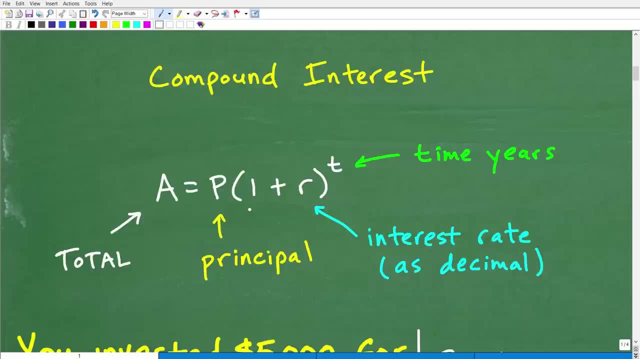 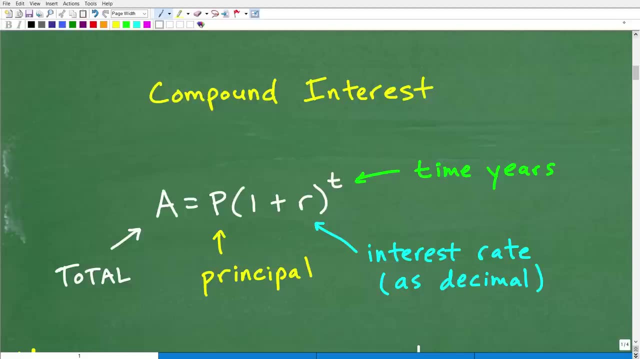 there's a compound interest that can be, um, uh, you know, quarterly or biannually, and those are for additional prompts. So this is kind of a basic introduction prompt. So here is the nice, lovely formula that we need to know for annual compound interest. So it's this: a is equal to P times one. 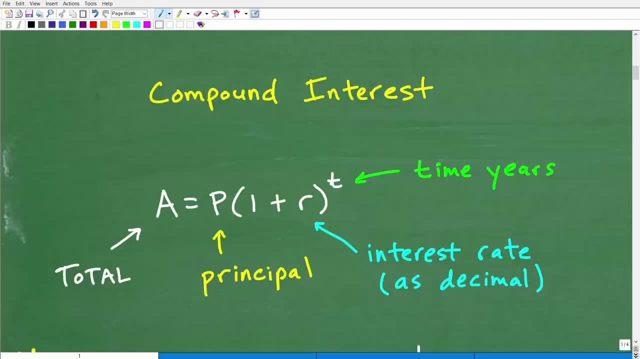 plus R. all that to the T power. So let's go ahead and talk about what these variables mean. And so a is your total amount of what you're going to make in your investment. Okay, So we're going to need to invest some money in that money is what we call a principal amount. Okay, So this is in. 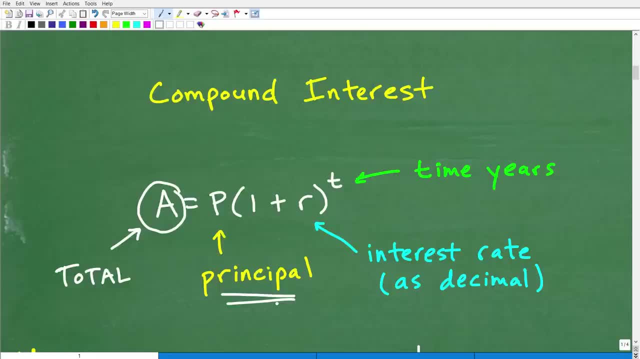 this particular problem. it's $5,000.. That's what we invested was $5,000.. It's our initial amount that we're going to invest. Uh, so that would be our principal amount. That's what P is. So we have parentheses, one plus R. now R is the interest rate. Okay, In this particular. 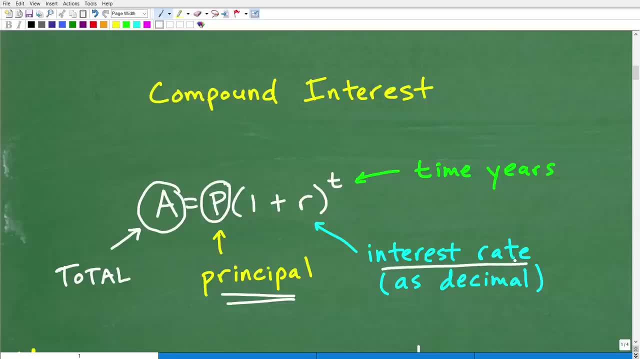 problem. it's 6%, It's the, it's the rate of a compound interest, And we're going to represent that as a decimal. Okay, So that's what R is, And then T is the number of years our investment is. 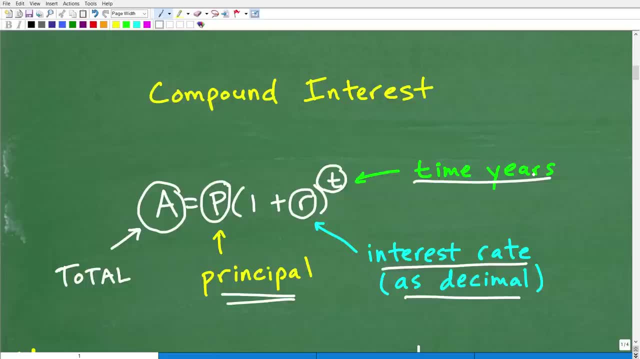 going to grow. Okay, So we're going to invest $5,000.. So we're going to invest $5,000.. And we're going to invest $5,000. Okay, So, if you kind of understand this, you're like: all right, you could. 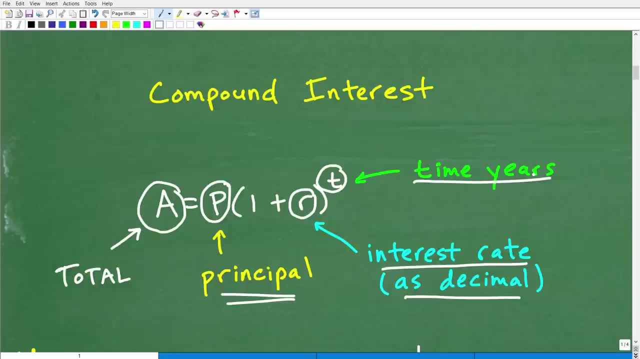 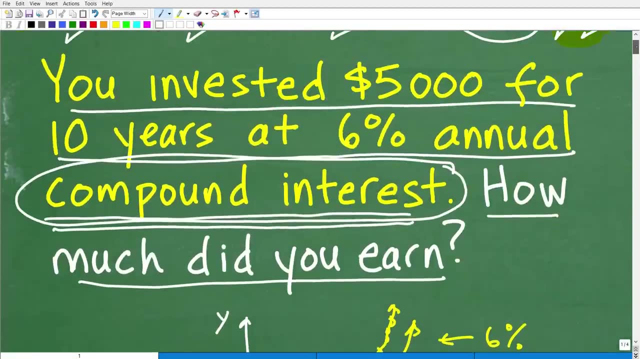 kind of you know, think about, you know, uh, this formula, Uh, this is not that difficult. If you're like, if you want to write this down and give this problem another try, let me show you the problem here. Go ahead and pause the video and see if you could do this. If you have a calculator, just be. 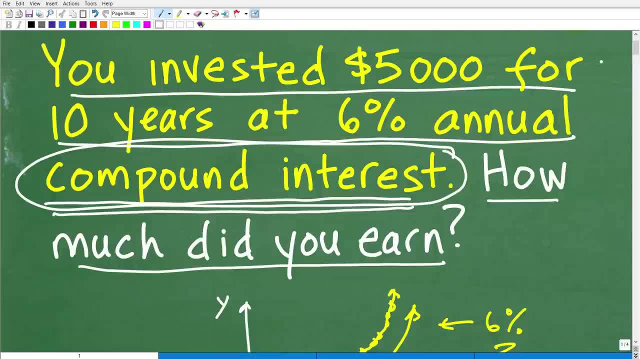 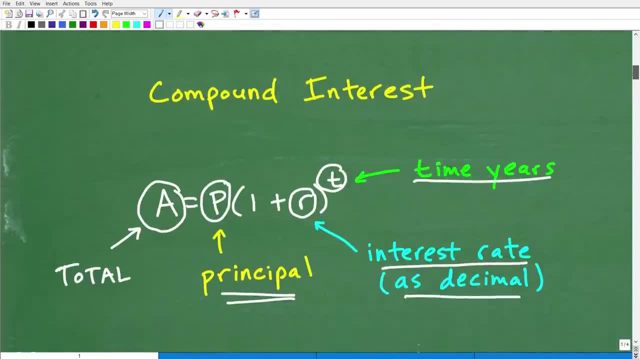 careful with the math because you know it's easy to make a mistake. I'll show you um a common place where students make an error. but you know, give this a problem and give this a try If you think you can, if you're like far enough into this video and you're like hell. 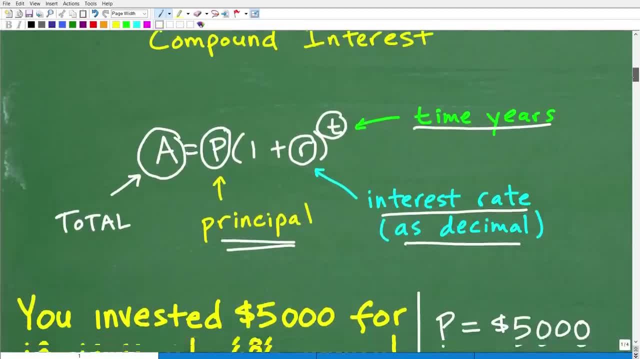 I get this now, then you should stop and see if you can do it, But anyways, let's go ahead and get into the actual solution right now. All right, So here's the problem. You invested $5,000 for 10. 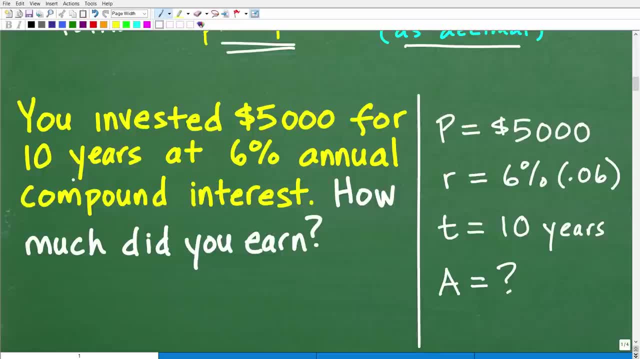 years at 6% annual compound interest. So we've got to make sure we understand what is the principle, What is the rate, What is the time. So the principal amount is what you invest, right? So you invested $5,000. So P is going to be $5,000. So our rate is going to be 6%. That's our compound. 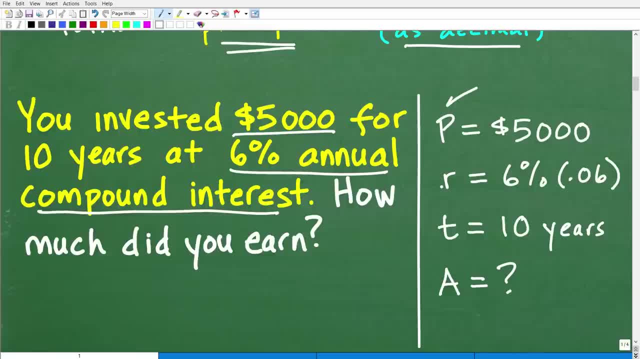 interest. So that's our compound interest. So that's our compound interest. So that's our interest. So that's our compound interest. So that's our compound interest. So that's our compound interest rate. okay, Our rate of growth, So that's what R is going to be. It's R is going to be. 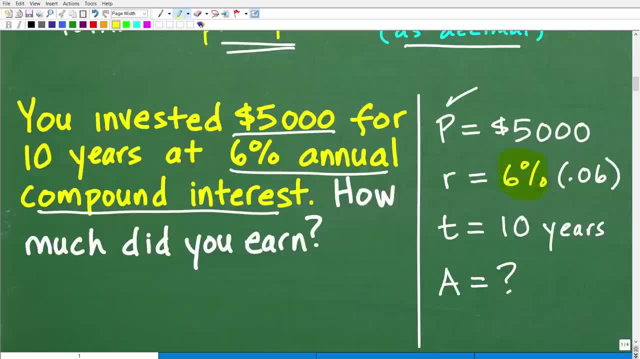 6%, But we're going to express this percent as a decimal. So how do you change a 6% to a decimal? Easy, You simply divide by 100 or you move that decimal point over two places to the left, So 6%. 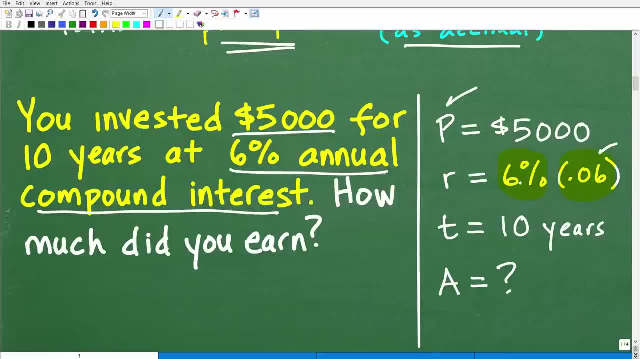 is 0.06.. So we're going to need the 0.06, not the 6%. And then the time is what? 10 years. So that's going to be 10 years, And what we're looking to, you know answer is: how much did this investment? 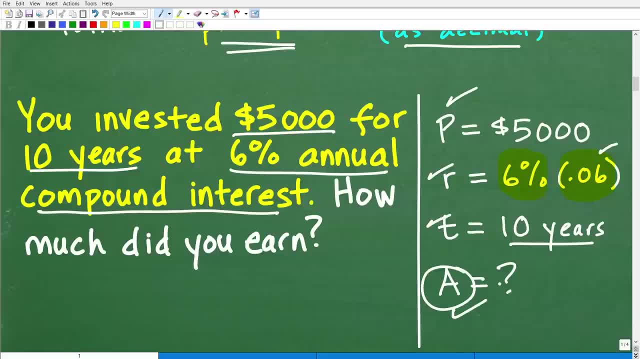 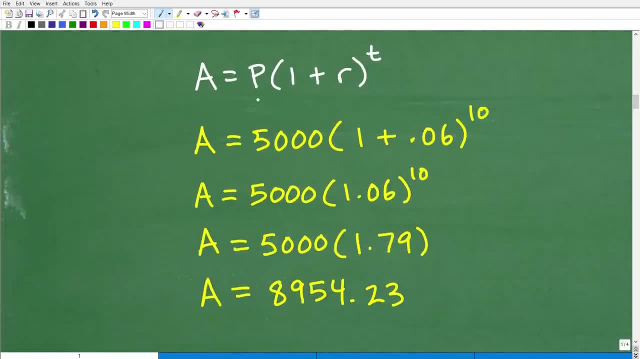 grow. So that'll be our total amount A. Okay, so let's just go ahead and plug this stuff in to the formula and we'll get the right answer. Okay, so P again is going to be 5,000.. That's going to. 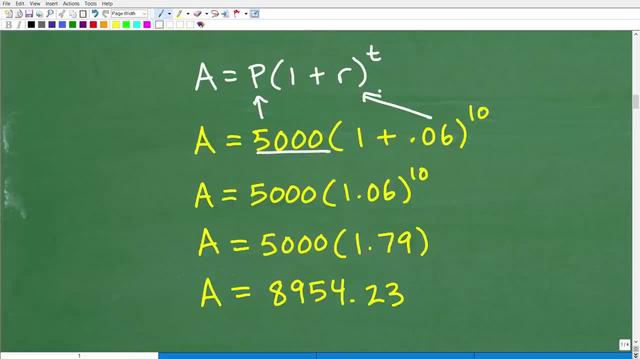 be our principal amount. So 1 plus R. R is our growth rate, our compound interest rate as a decimal. So 6% as a decimal is 0.06.. And T is going to be 5,000.. So that's going to be our. 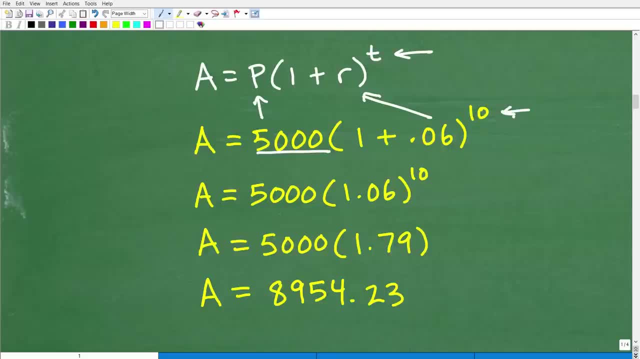 10 years And we have a 10 right there. Okay, so you got to be very careful here. You got to figure out what the order of operations is, So let's go ahead and do what's inside parentheses first. So 1 plus 0.06 is 1.06.. And that's going to be to the 10th power. Now here is where a lot 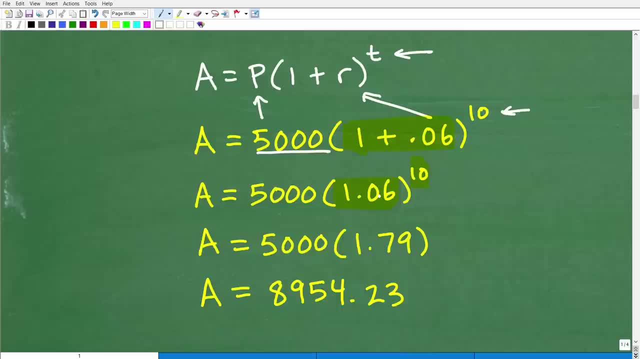 of students they do this part right, They get everything right. But I've seen this time and time again from like great math students in Algebra 2, college algebra, even pre-calculus. They kind of lose their mind. Maybe their cell phone, they get a text notification, or maybe their good friend. 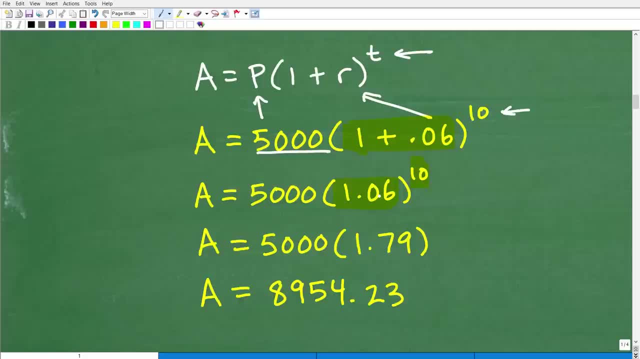 next to them says: hey, what's going on? They get distracted just like driving a car and they stop thinking for a second And what they'll do is they'll take this 5,000 and they'll multiply by 1.06.. Okay, I know they know better, but just to make sure you understand, this is multiplication. 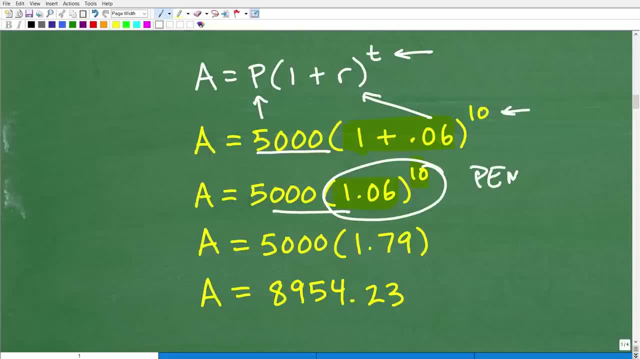 This is powers. Okay, so when we're talking about the order of operations, right, we did what's inside parentheses first. We did what's inside parentheses first. We did what's inside parentheses. first You got to do exponents or powers. next You got to take 1.06 to the 10th power. You got to. 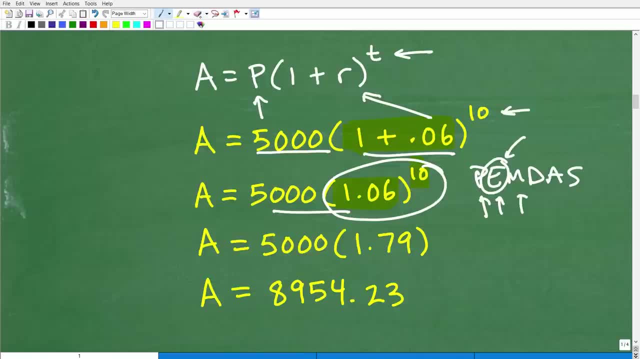 do that before multiplication and division. But you know, as a teacher you see some crazy stuff over the years. You know, again, I've been teaching math for not years but decades. Okay, so that means I probably looked at maybe 100 million different homework quizzes, maybe not. 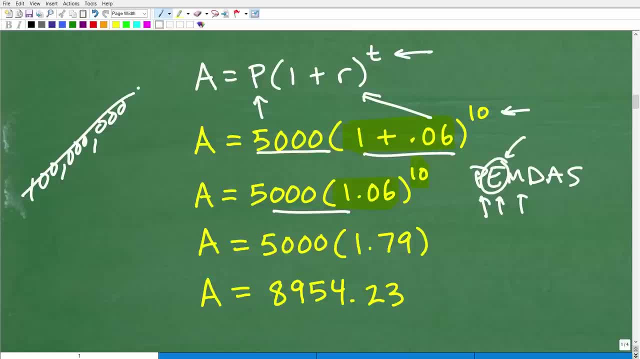 that many, but you get the idea a lot Okay. so you just see these trends, even with excellent math. So just you know, when you're doing any math problem you've got to remain highly focused until you get the final answer right. So anyways, we got to figure out what 1.06 to the 10th power 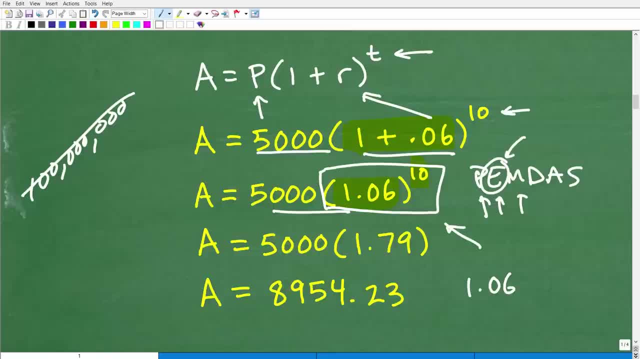 is on our calculator. So you just go 1.06, use that caret function- most of your calculators- to the 10th power And when you do that you'll get 1.79.. Okay, and notice how I'm showing all my work. 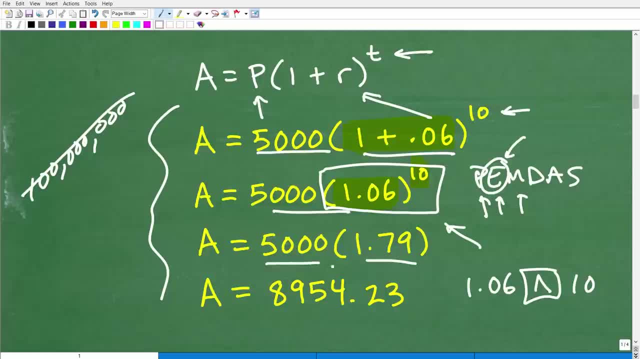 like this. This is what you need to be doing as well. Now. we can take that 5,000 and multiply by 1.79.. Okay, so you know, when you're doing any math problem, you've got to remain highly focused.